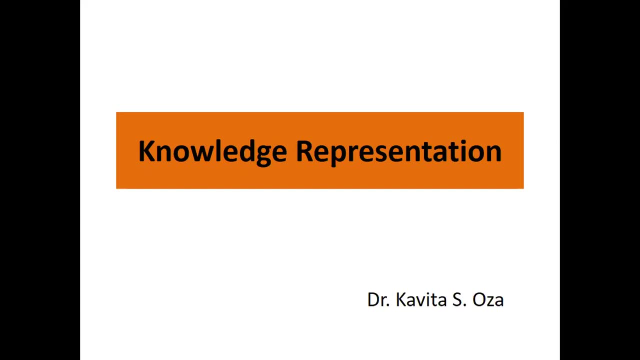 by giving them artificial intelligence right Now. to make machine intelligent, we need to make machines knowledgeable. Some knowledge should be given to the machines. that means they should build up their own knowledge base Now. for machines to become intelligent, you need to give them knowledge in the way they can understand. So there's a big whole thing. 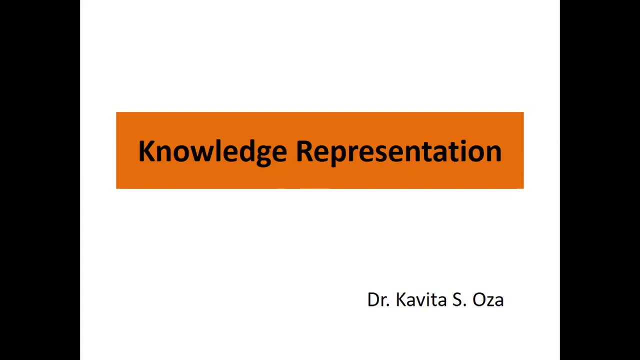 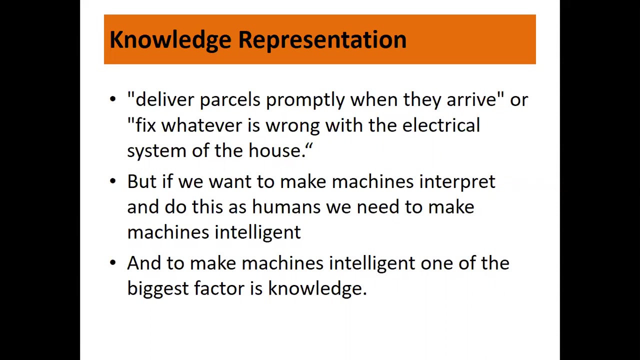 what is there behind how you represent a knowledge so that machines can become intelligent? So the second unit is totally based on knowledge representation. So let us start So, deliver parcels promptly when they arrive or fix whatever is wrong. Let us start with the electrical system of the house. These are the instructions. if you 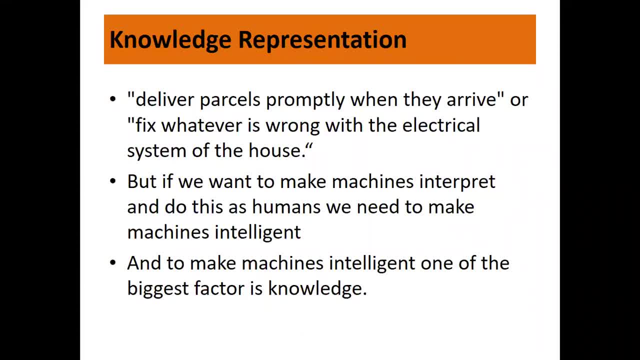 give it to the human being. they understand, they interpret and they work accordingly. But if you want to make machines interpret and do this as humans, we need to make machines intelligent Now. to make machines intelligent, one of the biggest factor is knowledge. See, 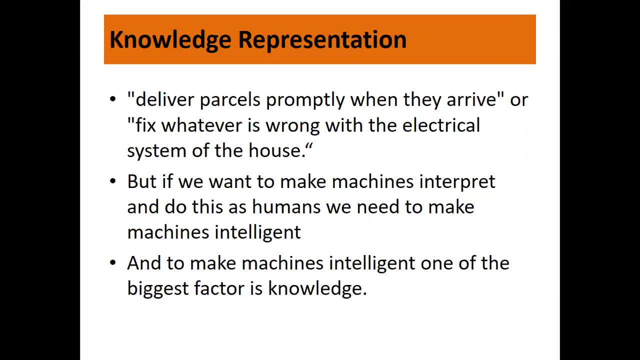 unless and until you have knowledge, you cannot do anything. If I want to go from one point to another point, let's say from one city to another city, I should know how do I go there? The paths available, the routes available. So the paths and the routes which are available. 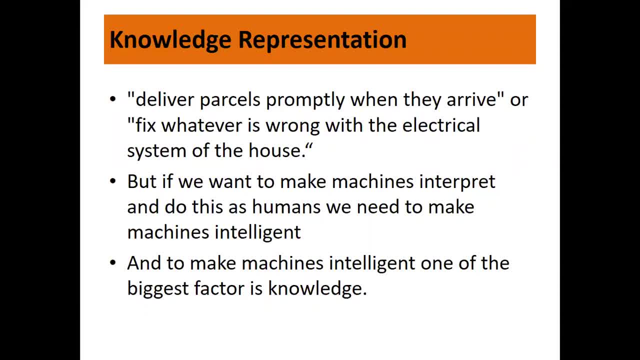 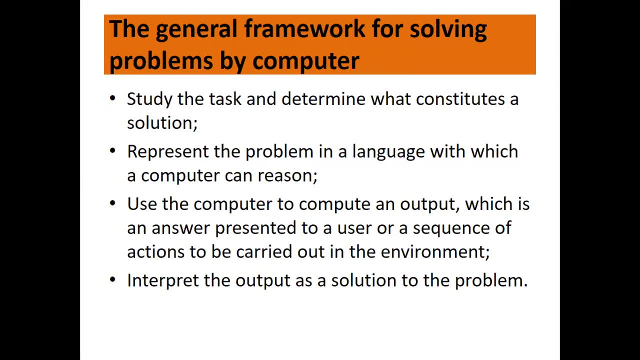 is the knowledge, but selecting a proper path to reach there is the intelligence. So how do computers solve a problem? What is general framework? You start, study the task and determine what constitutes a solution. If you want something to be solved by a computer, the very first. 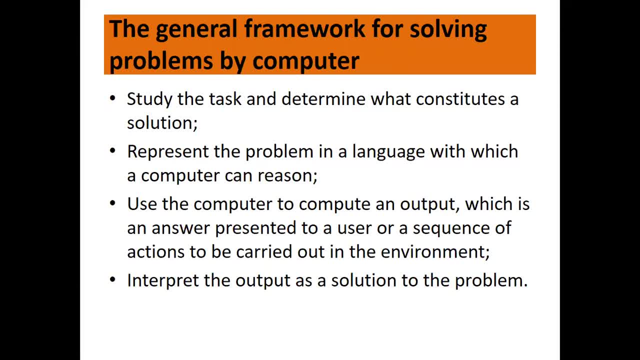 thing is study the task and determine what constitutes a solution. Represent the problem in a language with which a computer can reason Means whatever problem you want to get it solved. it should be represented in a way which computer can understand so that it can analyze the problem. Use the computer to compute. 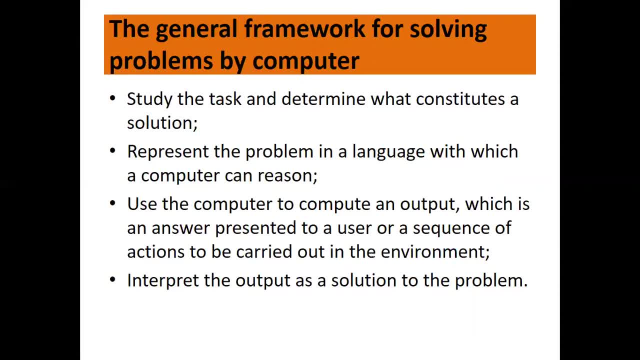 an output which is an answer presented to a user or a sequence of actions to be carried out in the environment. So what we do: once we know the problem, you analyze it and then you carry out the computation, and the output of the computation is a solution. What the 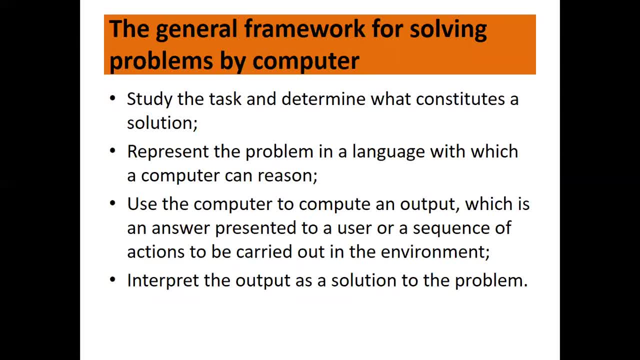 computation may be a single, maybe an answer, or it may be a sequence of actions to be carried out. Now. interpret the solution as a solution. interpret the output as a solution to the problem. This is a general strategy. what is used for solving a problem by computer? 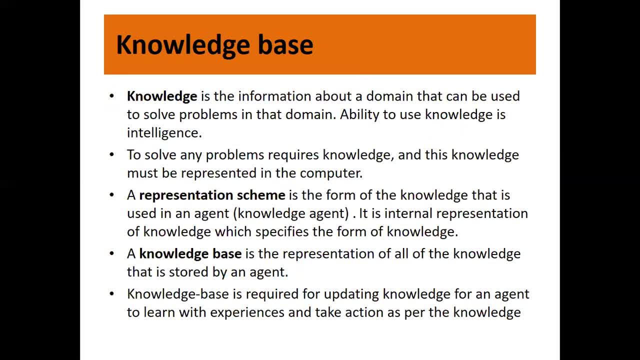 Now, as I said, knowledge- knowledge base- is an important term, what we'll be using throughout this unit. So knowledge is the information about a domain that can be used to solve problems in that domain. Now, ability to use knowledge is an intelligence, As I said. when you want, 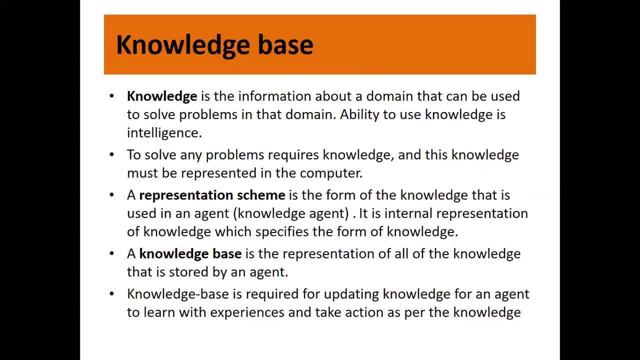 to move from one city to another city. there are so many ways, like you can go by train, you can go by flight, you can take your own car. There are many ways, but depending on how fast you want to reach, how urgent the work is, how much money you can spend you. 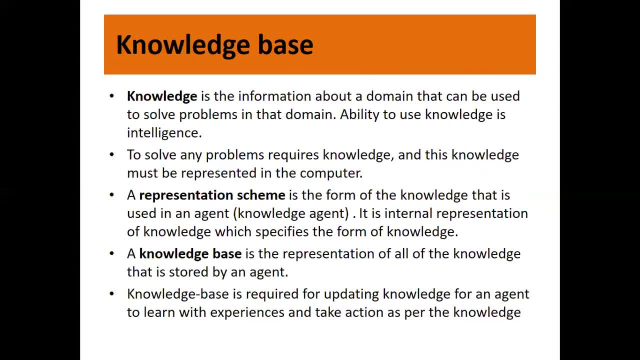 decide, and that is nothing but the intelligence. You decide the path, which path you need to take, and that is nothing but the intelligence. To solve any problem requires knowledge. You need to have knowledge, and this knowledge must be represented in the computer, because 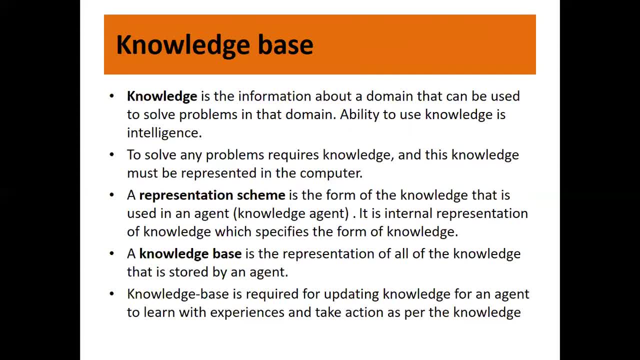 you want computer to solve the problem. A representation scheme is the form of the knowledge that is used in an agent that is knowledge agent. It is an internal representation of the knowledge which specifies the form of knowledge. So whenever you want to store, 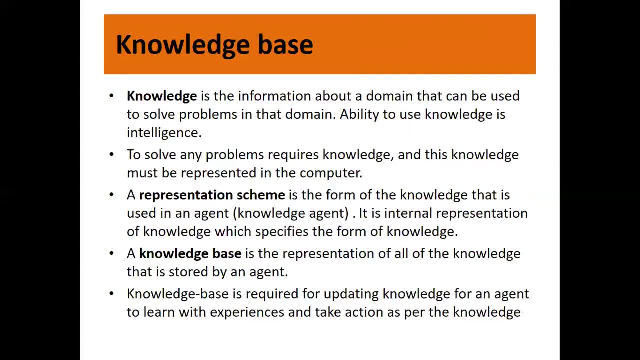 you want to make machines and intelligent, you need to give them knowledge. And for machines to understand the knowledge we need to have some scheme of representing knowledge. So in the knowledge right And once the scheme is ready, the machines can have their own. 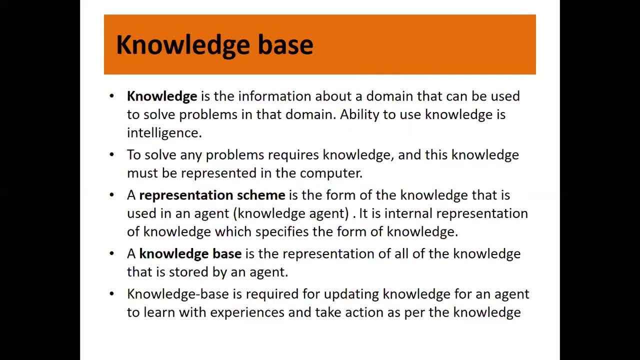 knowledge base. So knowledge base is the present representation of all the knowledge that is stored by an agent. Fine, A knowledge base is the representation of all the knowledge that is stored by an agent, And knowledge base is required for updating knowledge, for an agent to learn with experience and take actions as per the knowledge. 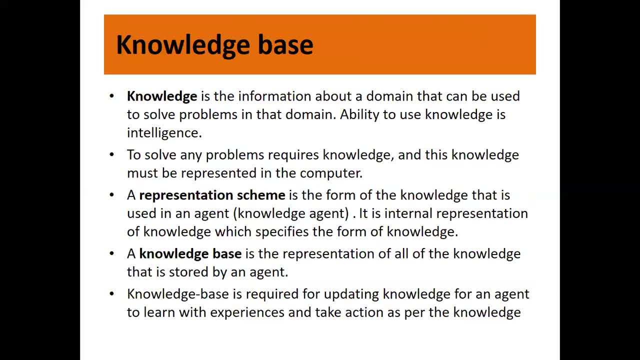 A simple example: if you take a chat bot right Once I fire a question, what chat bot will do? it will check it with the FAQ. If it is not existing in the FAQ, it will learn. okay, this is something new, what has appeared and I need to learn about it, so that will. 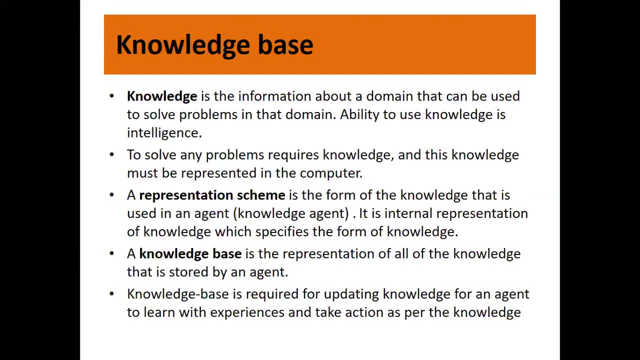 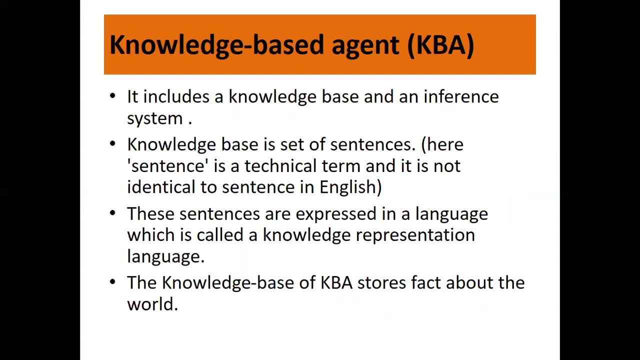 be added to a database and again it will be interpreted. So knowledge base is an important term. Now we have knowledge-based agents. Each of these agent will answer each question, So we are going to take a question question Now: what are these agents? They include knowledge base and an inference system. 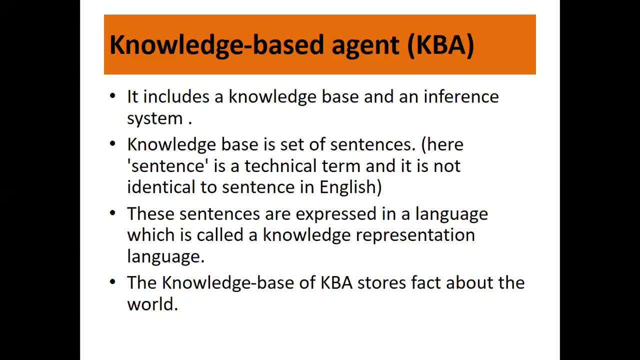 Now, knowledge base is nothing but is a set of sentences. Remember here, sentence is a technical word, It is not the sentence what we use in simple English when we are speaking and all. So these sentences are expressed in a language which is called knowledge representation language. 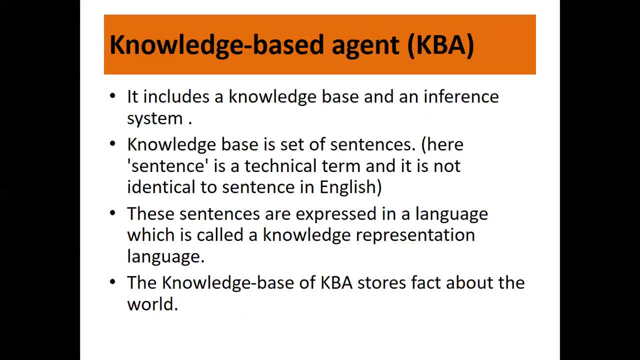 So these sentences are nothing but the input, what we are giving to the machine as a form of knowledge, And it should be expressed in a language what a computer can understand. See, knowledge representation is nothing but also structuring the data, What will be stored as a knowledge base in the computer? 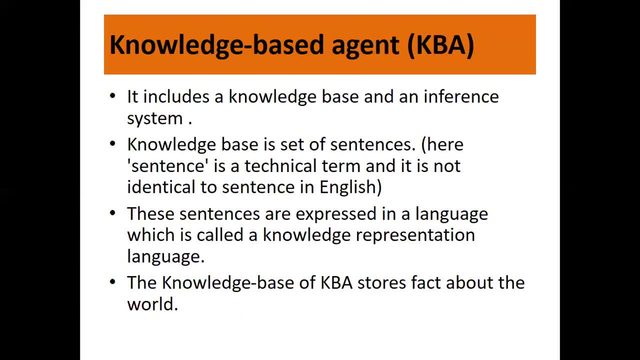 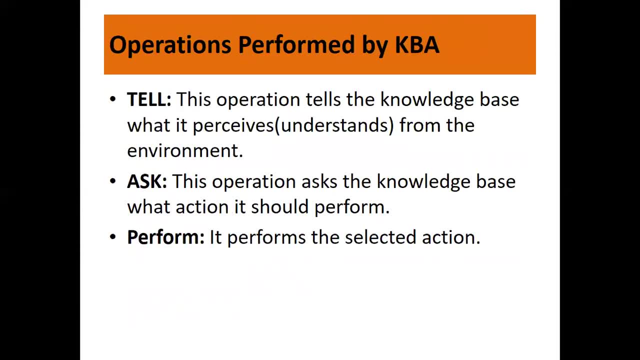 So the knowledge base of knowledge base agent stores facts about the world. Now, what operations are performed by a knowledge base agent? It has main three operations, that is, tell, ask and perform. So this operation tells the knowledge base what it perceives from the environment, what it understands. 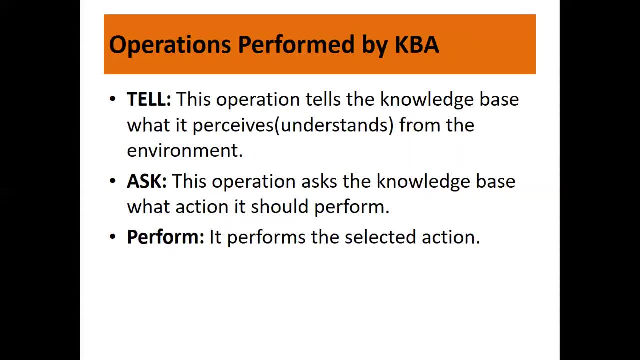 Ask this operation, ask the knowledge base what action it should perform And perform it performs the selected action. A simple example: again here we can take off a chat box, So chat bot, in fact. So once a question is given to the chat bot, 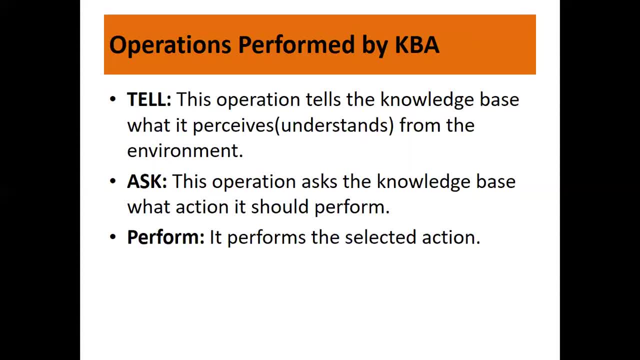 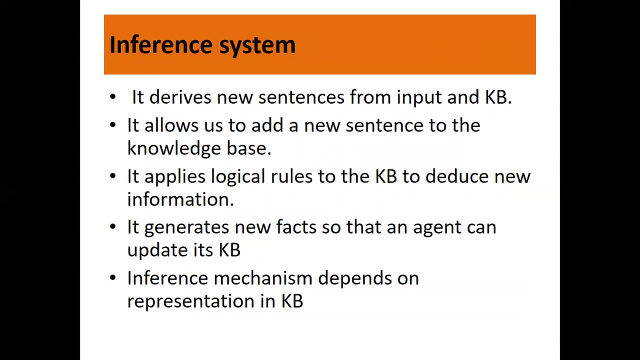 It will check, it will ask its data set whether the answer to this related question exists or not. If it exists, it will perform the selected action. Otherwise, it will give the message it cannot be done, Right? So what is the operation performed by your knowledge base agent? 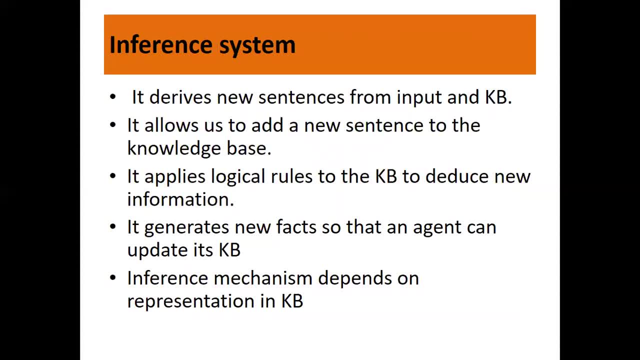 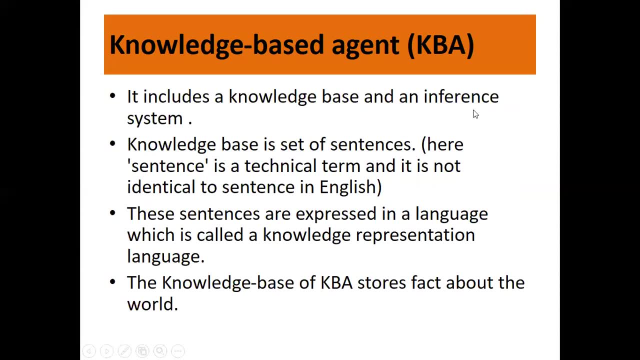 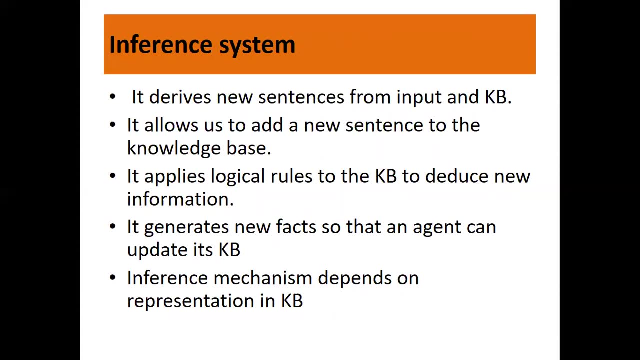 Now the second part is inference system. As we already know, What is knowledge base agent? It includes knowledge base and inference system. What is inference system? It derives new sentences from the input And knowledge base. It allows us to add a new sentence to the knowledge base. 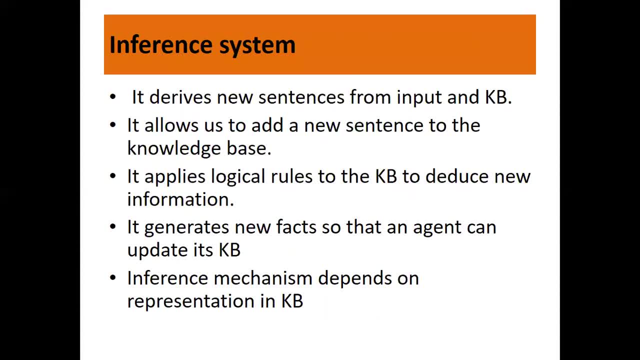 It applies logical rules to the knowledge base to deduce new information, Generates new facts so that an agent can update its knowledge base, And inference mechanism depends on the representation in knowledge base. So to understand all these things in a simple language, Again, let's go back to the chat bot. 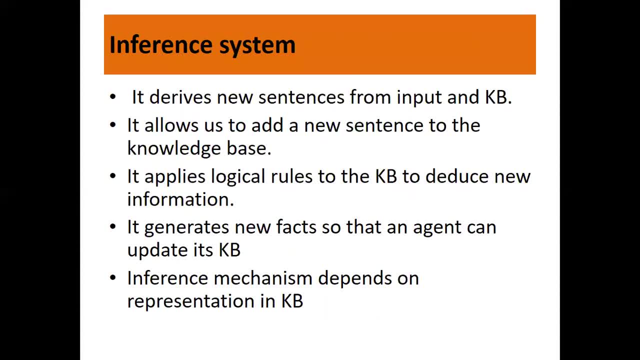 Right. When you are chatting with the chat bot, It derives new sentences from the input and knowledge base. So once I give a query, what I am asking or putting in the chat bot, What chat bot does, It will check it with the FAQ. 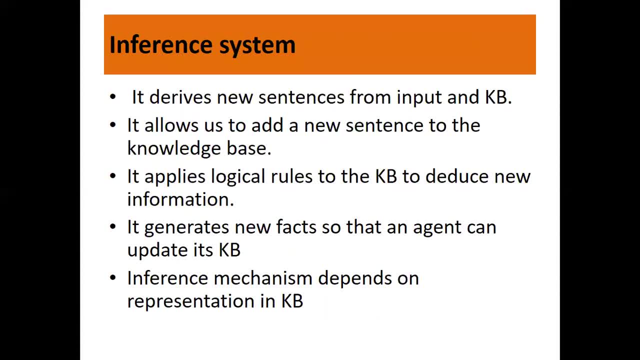 If it does not exist, that means it is a new sentence, what I have given Right? If it does not exist, it will add it to its knowledge base. That is something new has been added, So it allows us to add new sentences to the knowledge base. 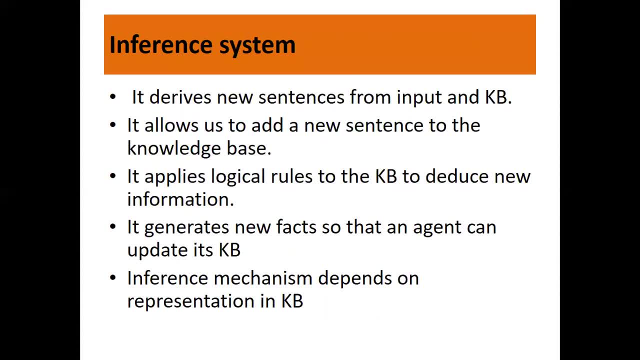 It applies logical rules to the knowledge base To deduce new information. Now, if something new is asked, Then it will try to get something from this knowledge base- Something related, not exactly- And come up with a new information. It generates new facts so that an agent can update its knowledge base. 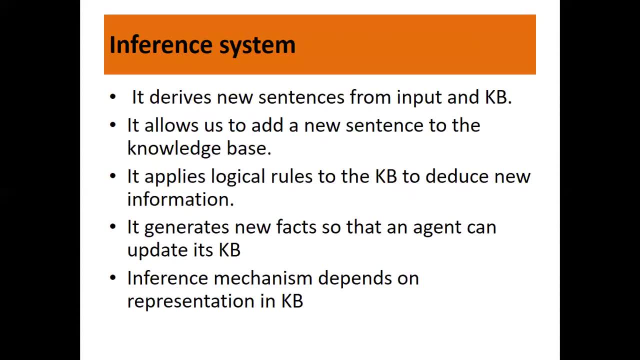 A simple example: if I have a chat bot And the chat bot is for MCA course or MSE course, The example will be when I am asking like about the fees. There may be many ways of asking In. the first way is asking: how much is the fees for MCA course? 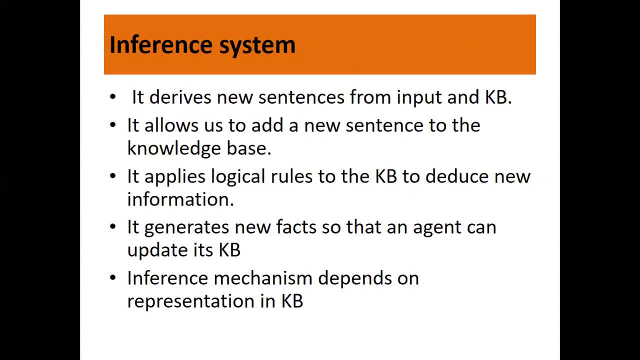 Second may be: just how much does MCA cost? Right, There are two different ways In my FAQ. if I already have the data stored, What is the fees for MCA, And when the question, the new input, what comes is how much MCA cost. 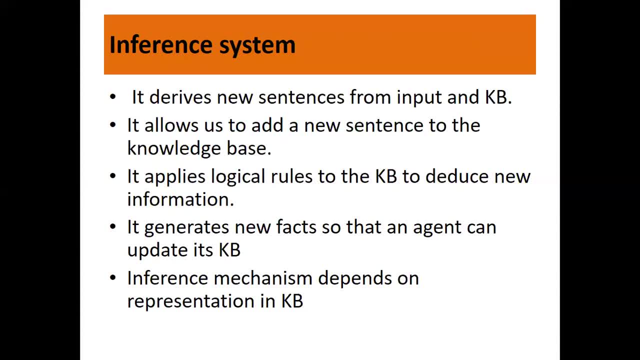 So, looking at the data base and the input, It should be able to interpret. okay, this is a query related to the fees And accordingly the result should be given. So inference mechanism depends on representation in knowledge base. How the knowledge is represented in a knowledge base plays an important role. 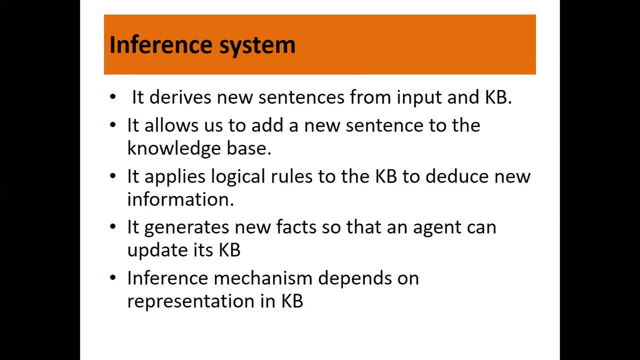 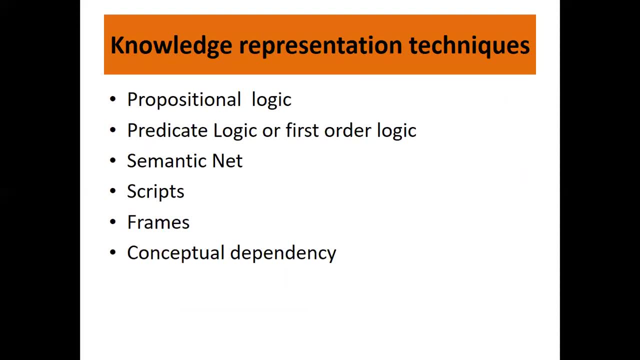 If the knowledge is stored syntactically, right, then you get the correct answer. So how many? there are different knowledge representation techniques. You have propositional logic, You have predicate logic or first order logic, Semantic net scripts, frames, conceptual dependency. 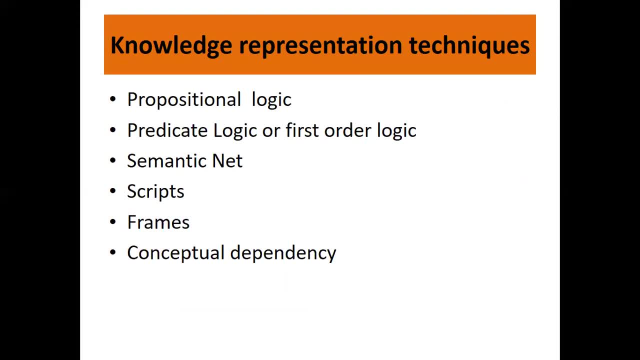 We look at them one by one in each lecture. Now there are inference techniques. There are three inference techniques. You have forward chaining, backward chaining and proof by resolution. As the name indicates, forward chaining is from the initial state of the problem to the solution. 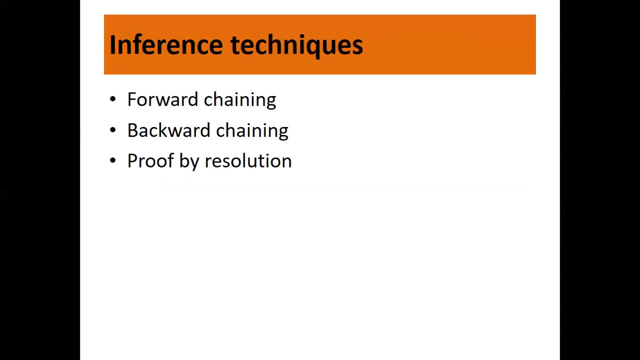 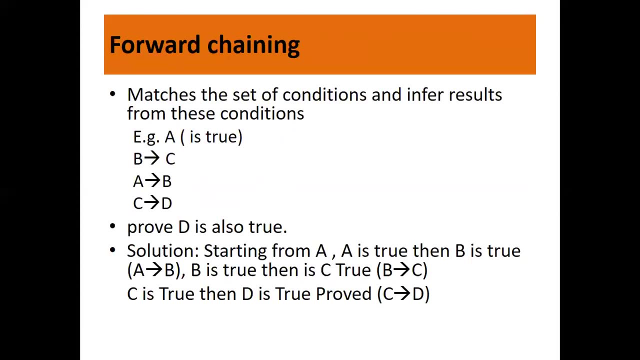 Backward chaining is from the solution, going back to the steps, what we have taken, And then what we have is proof by resolution where we will be using proposition logic, So forward chaining. simple example: it matches the set of conditions and infer results from these conditions. 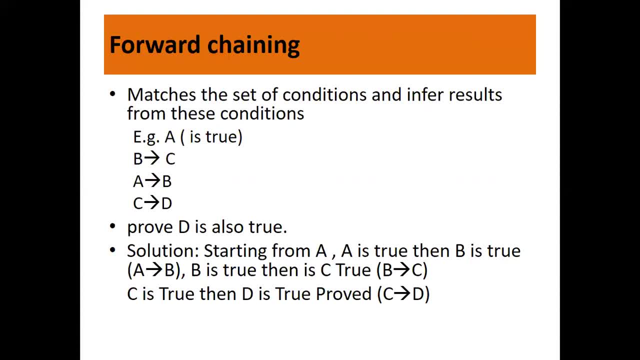 A simple example is taken: A is true and you need to prove B is also true. These are the rules given. So you start from A because A is true. You say A implies B. A is true, so B is true, B implies C. 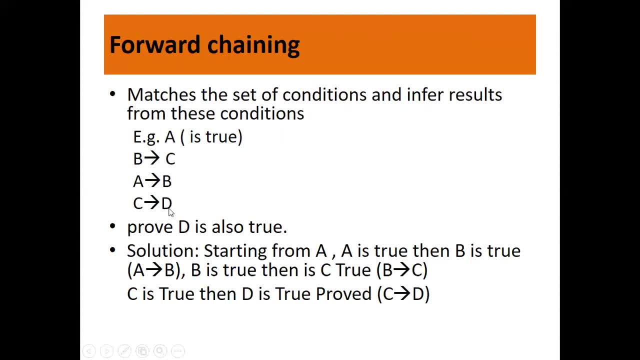 So B is true, therefore C is also true. And C implies A- D, So C is true, therefore D is true. That is D is true is proved. This is a simple example of forward chaining. The same example we will see how it works if you are using backward chaining. 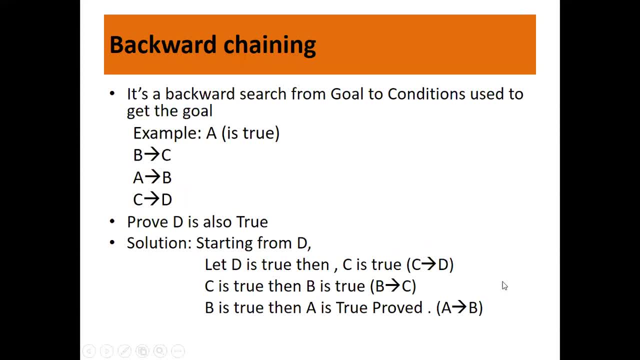 So, in backward chaining, the search is from goal to conditions used to get the goal. Again, you can see: A is true And these are the rules: what are given. What you need to prove, You need to prove. B is also true. So now, instead of starting from A, we are starting from B. 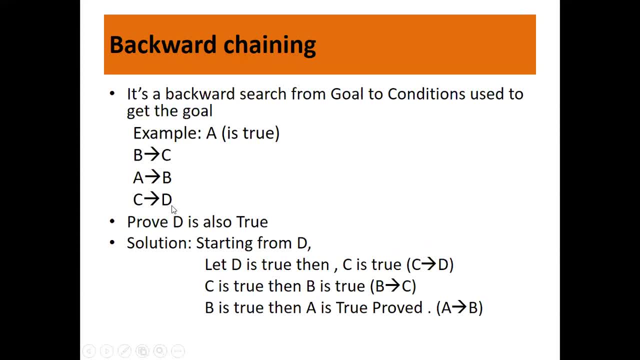 We know A is true, So we assume B is also true. When we assume D is also true, that means C is true. If C is true, B is also true. If B is true, then A is true. That means, starting from D, you can prove that A is true. 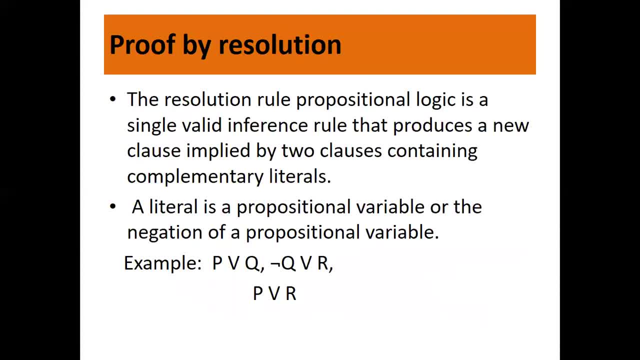 Very simple, it is a backward chaining. Now the next technique. what you have is proved by resolution. The resolution rule, propositional logic, is a single valid inference rule that produces a new clause implied by two clauses containing complementary literals. So what it is doing, 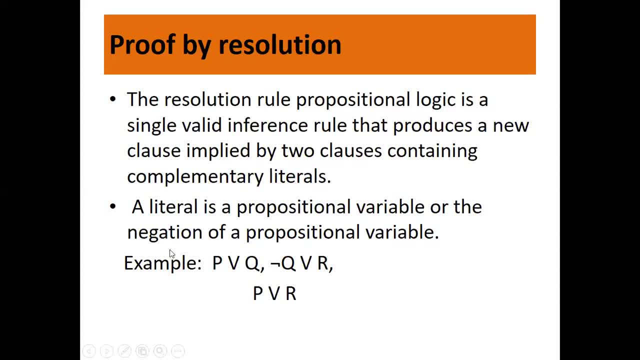 It takes two clauses and comes up with a new clause A, literal is a propositional variable or the negation of a propositional variable. Of course, you will understand better in the next lecture when we will talk about this. Right now, just remember P or Q. 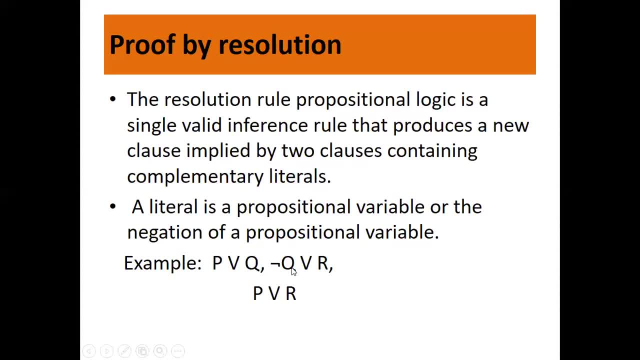 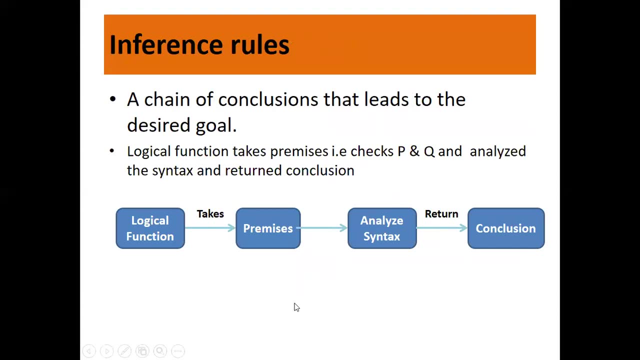 One literal Negation of Q or R, Another one. So what you get? the new literal. what is created is P or R. This is simple, proved by resolution. Now, what are the inference rules? It is a chain of conclusions that leads to the desired goal. 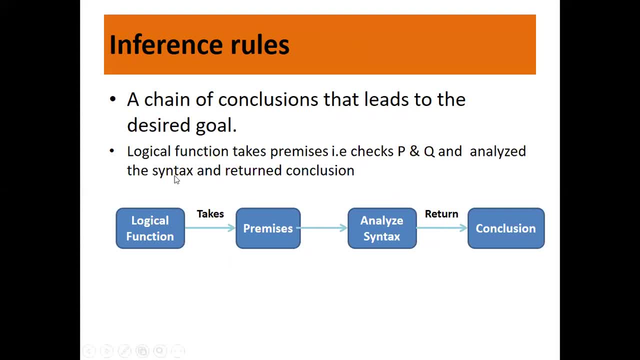 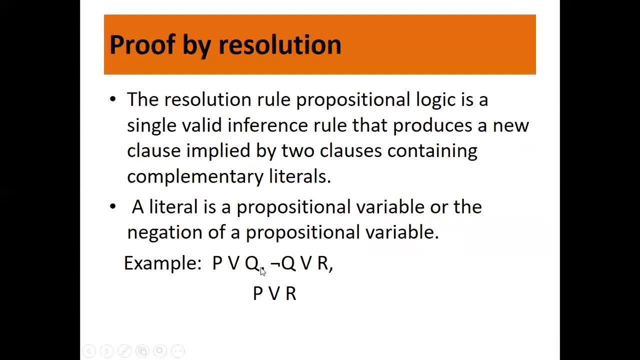 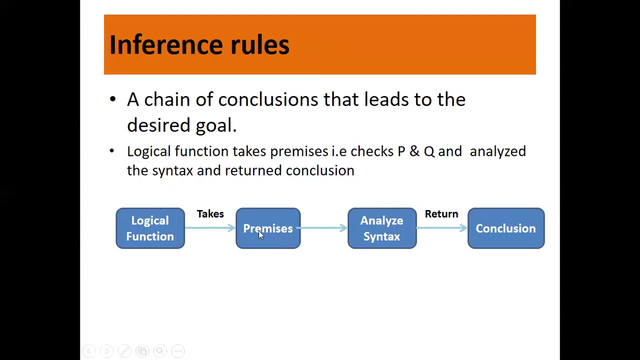 So logical functions takes premises, that is, checks P and Q, and analyzes the syntax and returns the conclusion. So if you take logical functions like here, if you look at this, P and Q, Fine, So it takes the logical function, takes the premises, in the sense it checks whether P is true or Q is true or they are false. 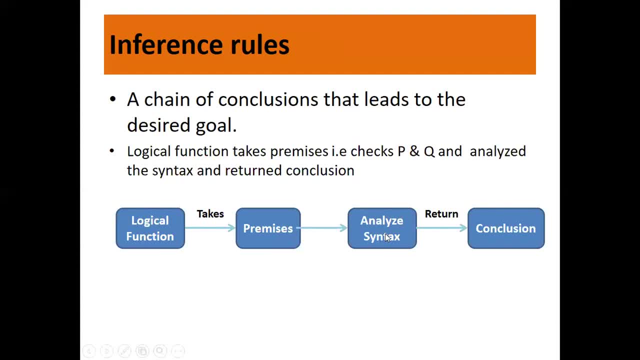 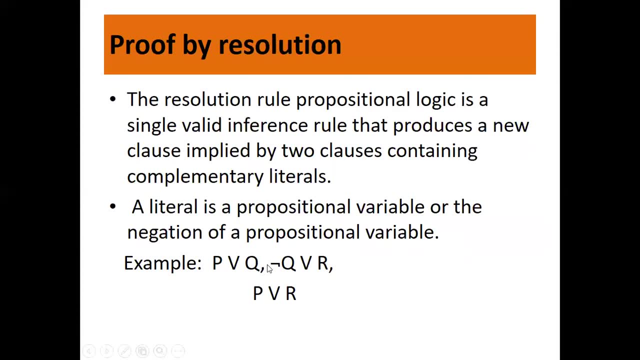 And analyzes And analyze the syntax, whether they are syntactically correct, and then returns the conclusion. If you look at it here, P and Q are taken, Q and R are also taken. They are analyzed whether the value is correct or no. 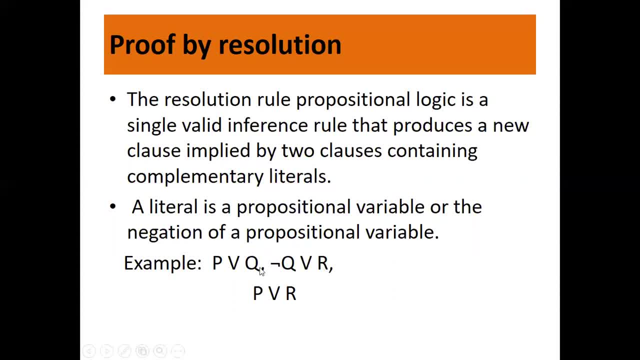 P is false or true. Now here, if you see, Q is true here, Q is false here, Negation of Q- And then it checks whether syntactically they are right or no, And then it analyzes, It gives you the conclusion. 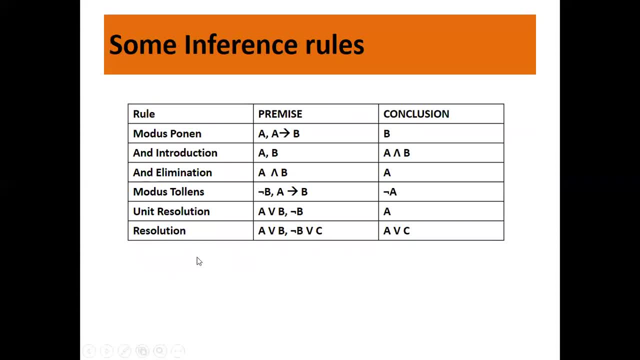 There is a simple inference rule. Now, these are some inference rules, what I think you should remember: Rules, premises and conclusion. You have modus ponens, You have AND introduction AND elimination, Modus tollens, Unit resolution And resolution. 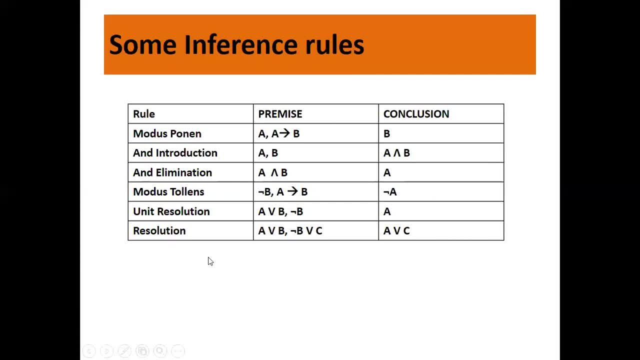 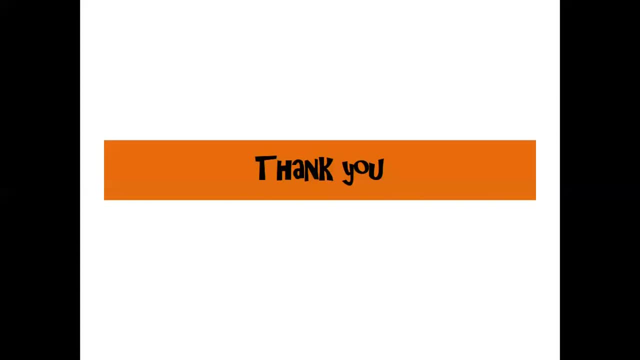 So this is the table, which will be very helpful for the reference as we go further. Thank you, I hope the simple concept of knowledge representation is clear. The overall summary of this presentation is: you want to make machines intelligent. To make machines intelligent, machines should have some knowledge base.